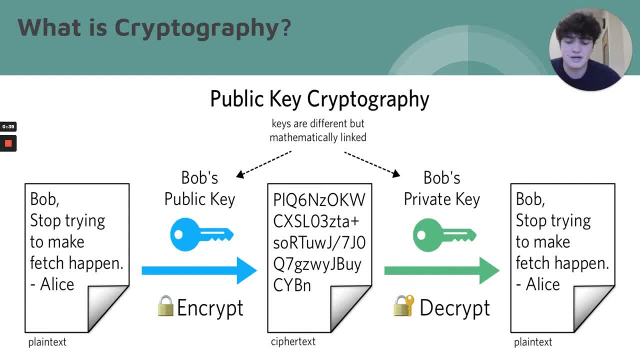 This is where cryptography comes to the rescue. Cryptography is the study of mathematical functions which are used to scramble information so they can only be interpreted by the intended recipient. In this way, our private information will appear meaningless to somebody who isn't meant to get their hands on it. 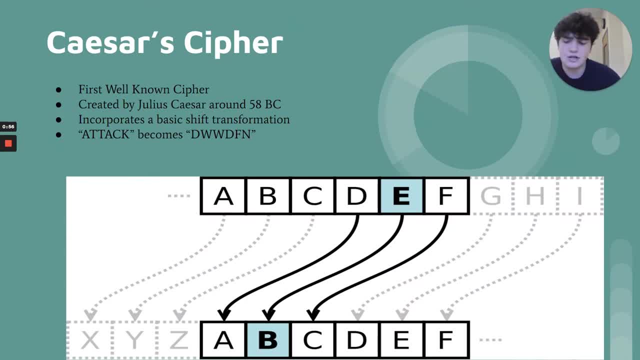 In order to better understand the explanation, let's take a look at the first well-known private key crypto system, known as Caesar Cipher. This cipher was first created around 58 BC by Julius Caesar, which he used to send encrypted messages to his military. 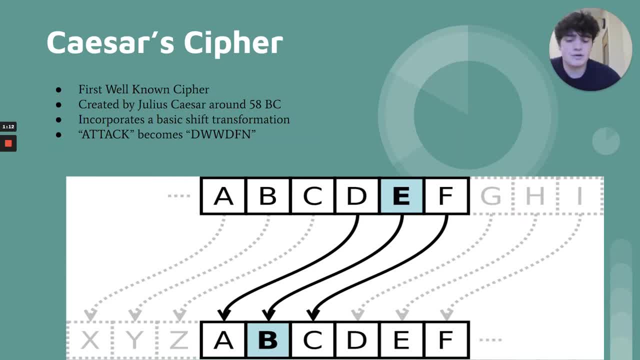 To encrypt his messages, Caesar simply shifted each letter of the original message three letters down the alphabet. For example, A became D, D became E, etc. By looking at the slide we see that if Caesar wanted to send the message attack, 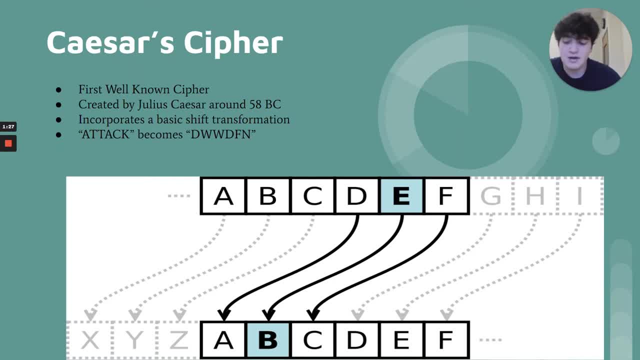 it would become D, E, etc. This means that if Caesar wanted to send the message attack, it would be D, W, W, D, F, N. Then the intended recipient of this message simply had to shift each letter of the enciphered message three letters back in order to recover the original message. 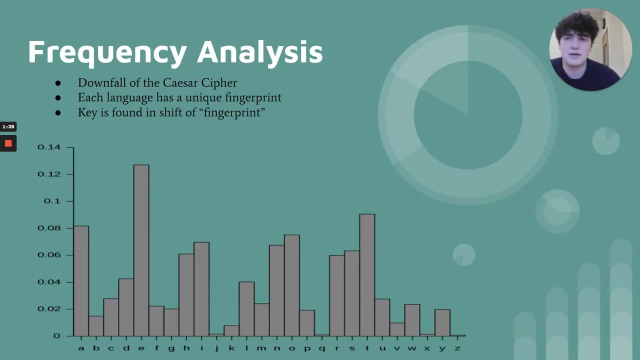 Surprisingly, this crypto system worked for hundreds of years, despite being extremely simple. Everything changed one day when an Arabic mathematician known as Al-Kindi used an important characteristic of the English language in order to break the Caesar cipher. This breakthrough was known as frequency analysis. 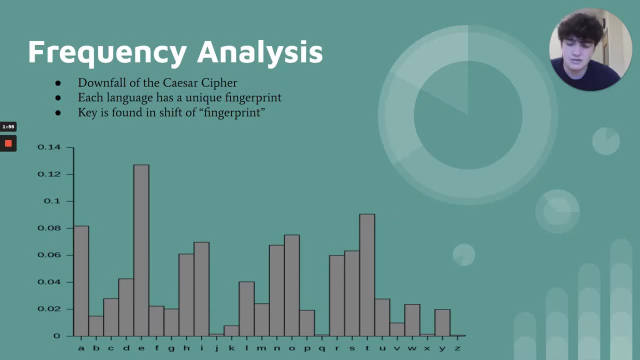 If you open any book or newspaper or lengthy text document and count the number of times each letter occurs, you will find a recurring pattern: E will occur more times than any other letter, while T will occur the second most, etc. This characteristic can be thought of as the fingerprint of the English language. 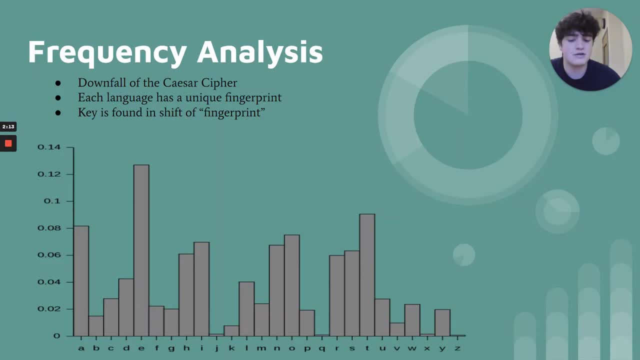 Al-Kindi recognized that if we count the number of times each letter codes in our ciphertext, which is our scrambled message, we simply need to count the number of times the most frequently occurring letter has been shifted down the alphabet. In other words, 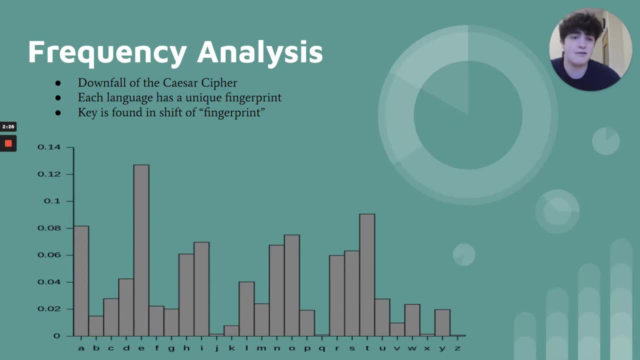 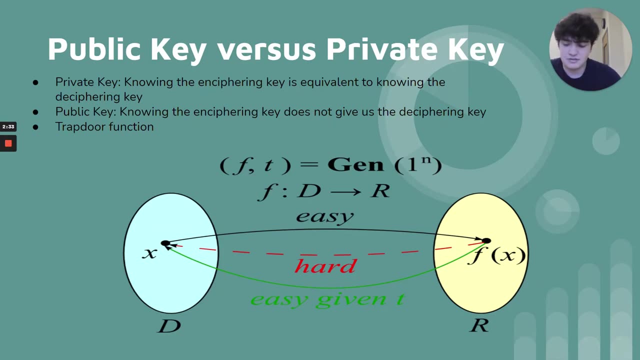 how many letters are fingerprinted. Our fingerprint has shifted down the alphabet and we have our deciphering key. The Caesar cipher is the most basic example of a private key crypto system. This is a crypto system in which knowing the enciphering key- in this case, 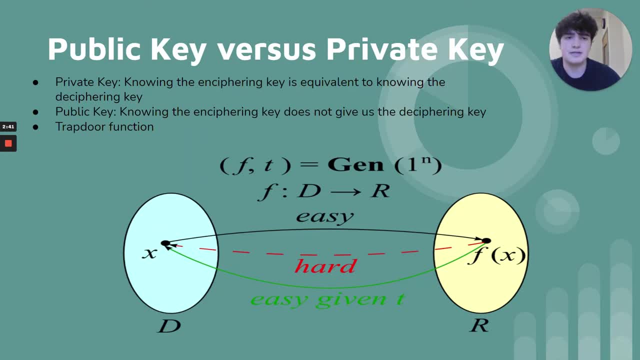 a shift of three letters down the alphabet allows us to determine the deciphering key negative three letters down the alphabet. It is not difficult to see where the problem lies with such crypto systems. We can decrypt the message by knowing either the enciphering key or by knowing the deciphering key. 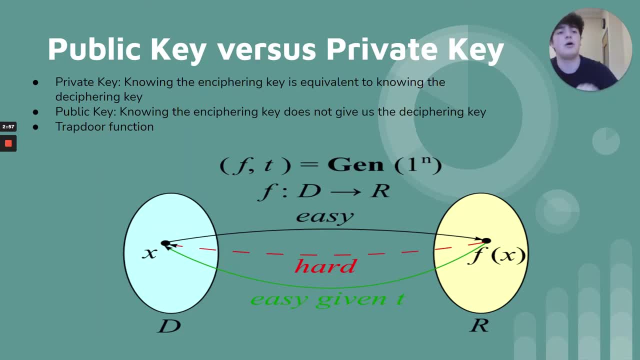 Additionally, both the sender and receiver would need to have agreed upon these parameters beforehand, which can be time-consuming and dangerous if the key were somehow to slip out into the public. It might be better if we had a crypto system where there was only one decryption key, and this is where public key cryptography comes in. 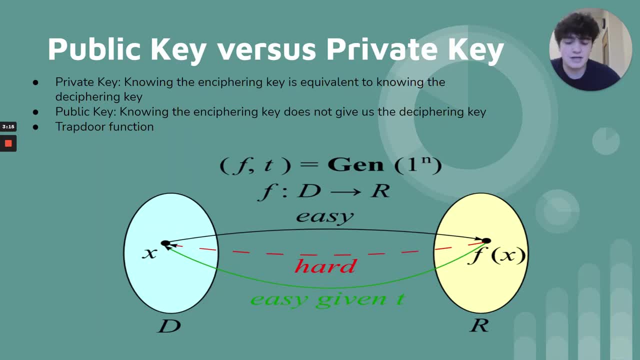 With public key cryptography, somebody who has knowledge of the public key cannot use it in order to determine the deciphering key. In other words, if Alice wants to send a message to Bob, all she needs to know is Bob's password, And then all Bob needs to do is use his private key in order to decrypt the message. 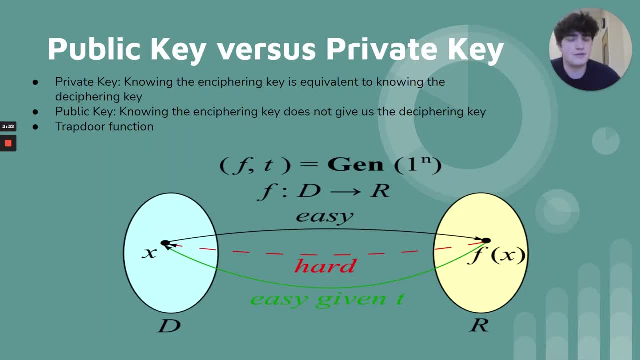 In this case, both parties do not have to agree on parameters beforehand, and so the process of sending an encrypted message is much more fluid and efficient. To do this public key cryptography makes use of a special mathematical function known as the trapdoor function. 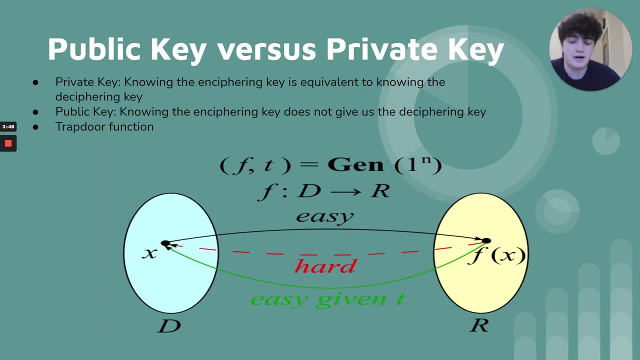 This is a function that is easy to compute, while its inverse is very difficult to compute. In cryptographic terms, this means that knowing the enciphering key makes it very easy for us to scramble the message, but trying to unscramble the enciphered message is extremely difficult. 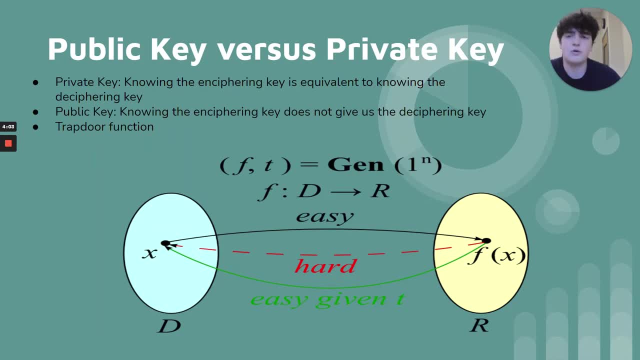 A good analogy in better understanding public key cryptography would be to think of the mailbox outside your house, Anybody can leave a letter in your mailbox, as it is accessible to the public, but only the intended recipient. you have the key to unlock the mailbox and read the mail. 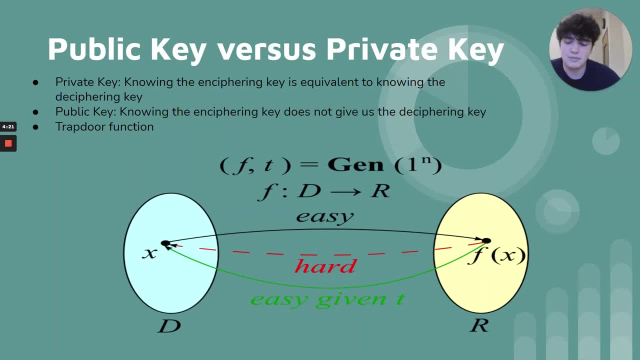 Public key cryptography allows us to more efficiently send information over public networks. because now, instead of having to use the cryptography, we can use the cryptography to decrypt the message. Because now, instead of having to use the cryptography, we can use the cryptography to decrypt the message. 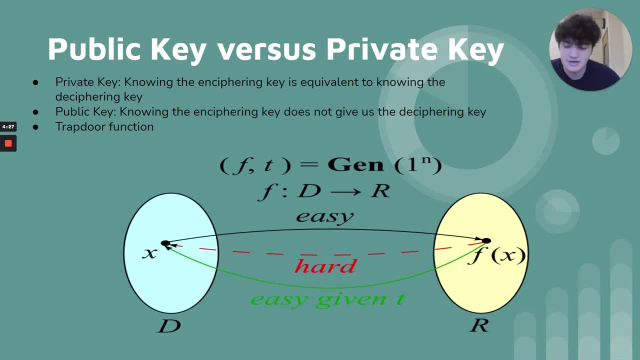 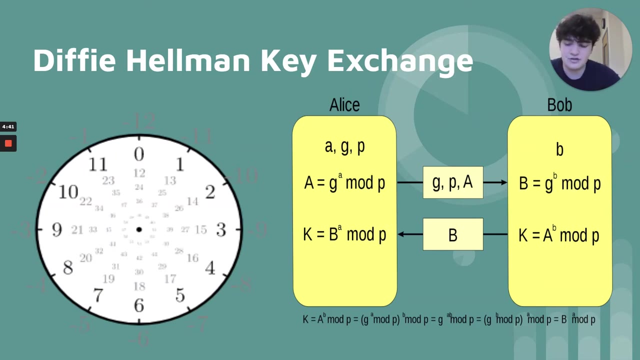 But instead of having to agree upon a certain key or go to lengths of exchanging keys, we can simply find anybody's public key out there in the public and send them a message that only they will be able to open with their private key. Let's explore the first example of a public key cryptosystem which is widely used today. 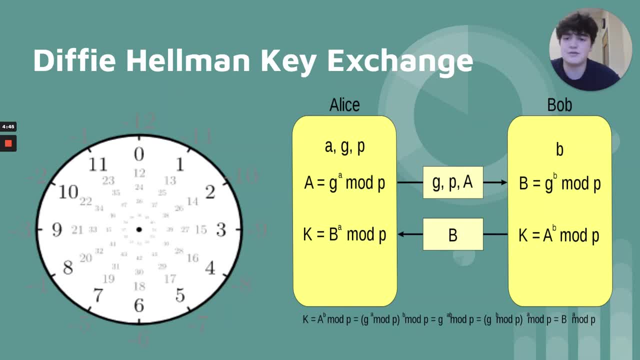 known as the Diffie-Hellman key exchange. But before we do so we need to develop a basic understanding of modular arithmetic. When we divide a number by another number- modulus N- we are finding the remainder after division. For example, by looking at the picture on the slide: say, we are modding by 12.. 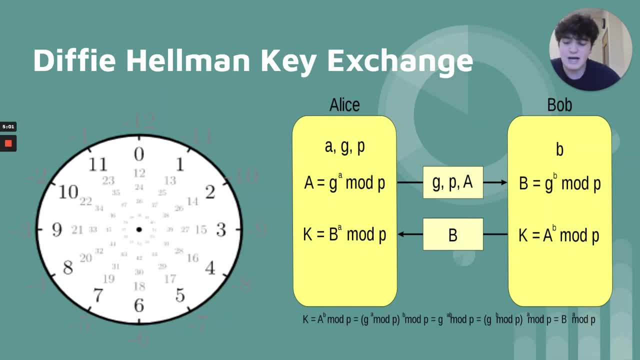 13 mod 12 is equivalent to 1.. This is the same as the hour handle of the clock, starting at 12 and moving 13 hours. Similarly, 12 mod 12 is 0,, 24 mod 12 is 0,, 18 mod 12 is 6, etc. 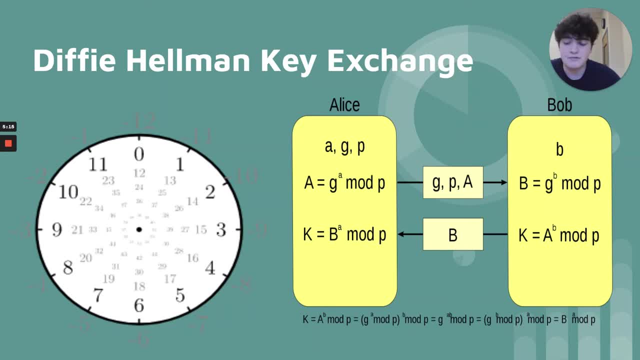 Cryptography uses modular arithmetic in order to bring an element of randomness into cryptography, as well as to limit the number of possible outcomes to a finite set of solutions, as computers are finite. Now let's suppose that Alice wants to send a message to Bob using the diffe-hellman-key exchange. in order to do so, Alison and Bob agree upon a modulus b. 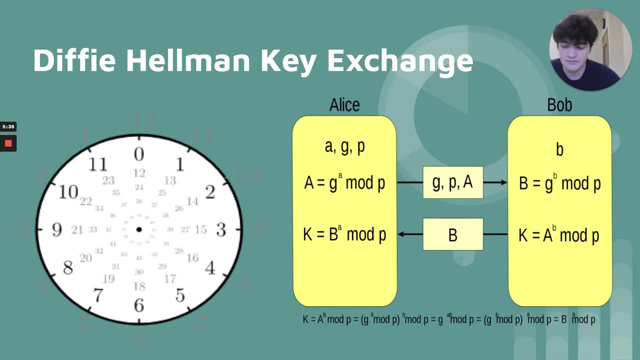 p, which once again can be thought of as the number of hours on the clock phase, as well as a generator, g, which is an element of the set of numbers 0 through p. Note that g and p are known to the public. Alice has her own private key, a, which she doesn't make known to the public. 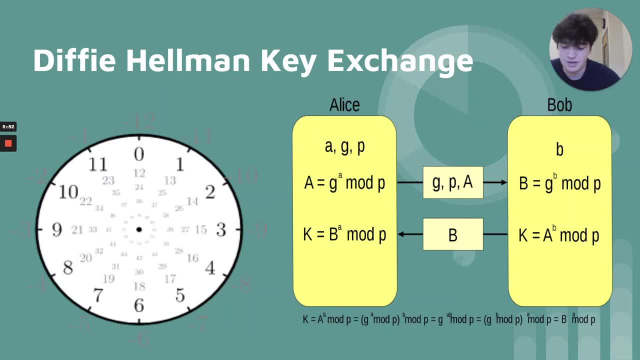 and similarly, Bob has his own private key b, doesn't make known to the public. Alice then takes the generator G and raises it to her private key A and mods the outcome by P. Similarly, Bob takes the generator G, raises it to his private key B. 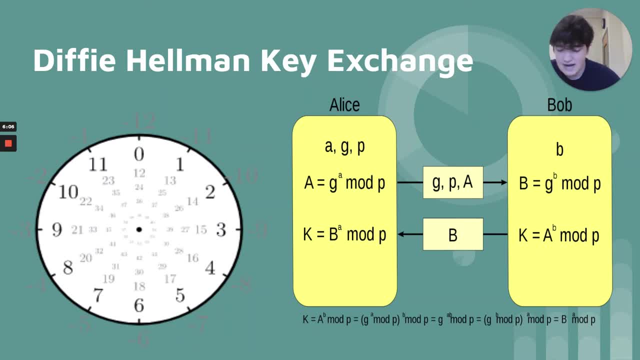 and then mods the outcome by P. They then send each other these values, which obviously means that they are made known to the public. Alice then receives Bob's the outcome. well, Alice then receives Bob's public component of the symmetric key and then she raises it to her private key A. 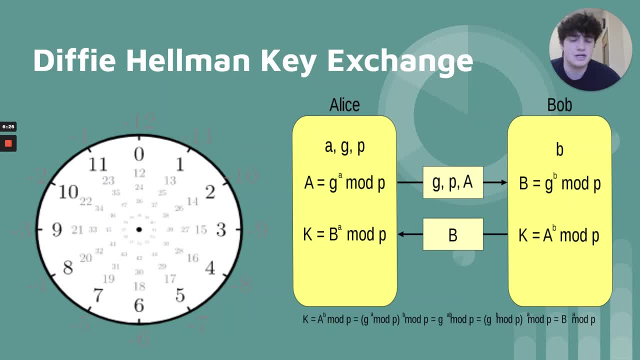 while Bob does the same, He receives her public component of the symmetric key and raises it to his private key B. Now they have both created the private symmetric key G to the A times B. In this way, Alice and Bob have essentially created a key together. Note that the trapdoor function is: 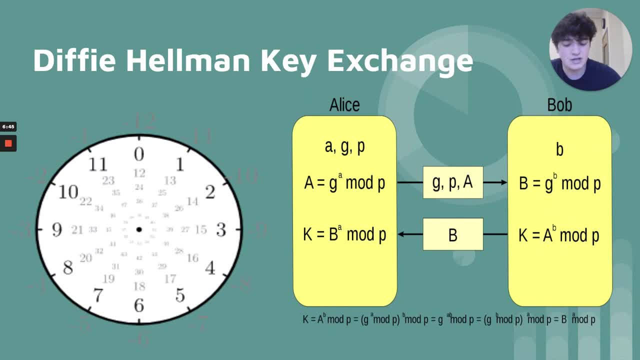 the reason that Diffie-Hellman works. When Alice and Bob send each other their public components of the symmetric key, a person that intercepts this value will not be able to extract Alice's private key A or Bob's private key B from it, as they don't know A or B, They'll never. 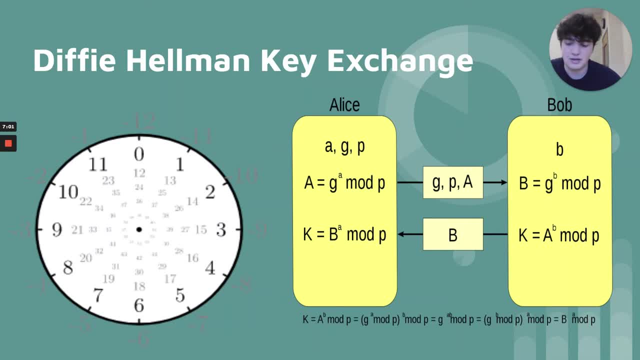 be able to know G to the power of A times B mod P. In other words, they'll never be able to access the deciphering key. To summarize, Diffie-Hellman key exchange is an encryption algorithm that requires both sender and receiver to participate in the creation of a mutual private symmetric key. 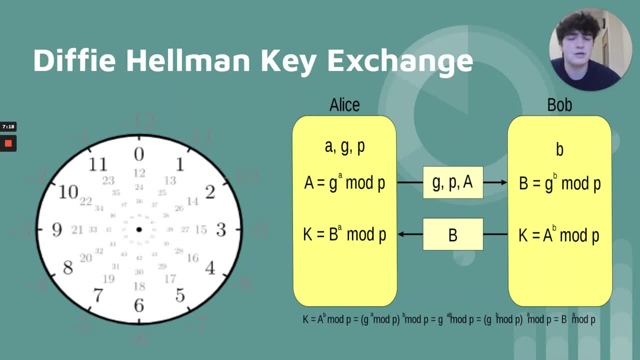 It's not hard to imagine, then, that the Diffie-Hellman key exchange will be able to access the different key pieces of the cryptography That Diffie-Hellman is used whenever people message each other over social media, because each participant is actively involved in the chat. 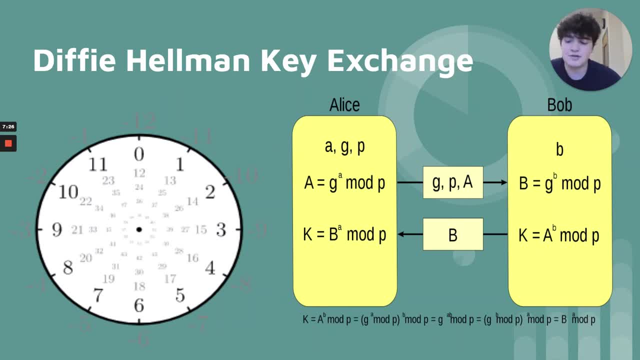 process. Additionally, we clarify that the main difference between private key and public key cryptography is that in public key, knowing how a message was encoded doesn't tell us how to decode the message, whereas in private key, knowing how to decode and encode the message are essentially the 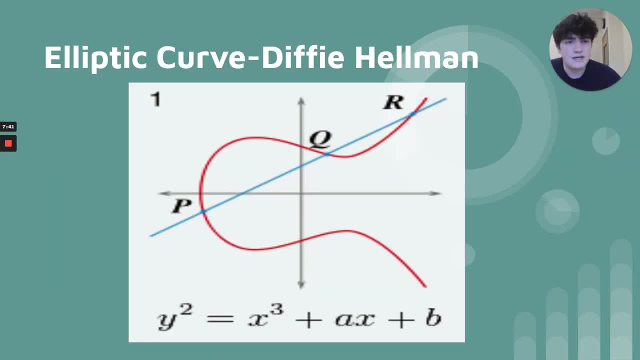 same thing In cryptography. since all computations are done on computers, mathematicians are constantly trying to find the key that the key will be able to access, the key that the key will be able to access, the more efficient ways to do encryption. In this section, we'll be talking about the elliptic. 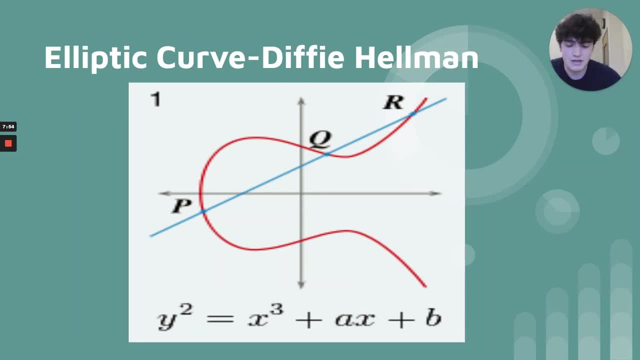 curve- Diffie-Hellman key exchange. So what is an elliptic curve? An elliptic curve is a curve in two dimensions defined by the function. y squared equals x cubed plus ax plus b. The coordinates along this function form the equivalent of the clock face values in the regular Diffie-Hellman. 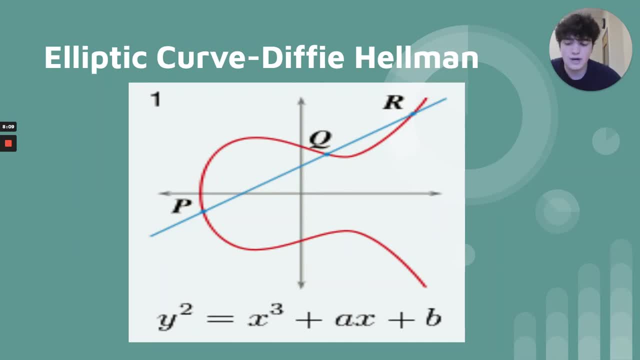 key exchange that we discussed before. In Diffie-Hellman we had that our generator and private keys, a and b, were elements in this number set 0 through p. but in elliptic curves our generators represent individual coordinates along the curve, while a and b represent natural numbers. 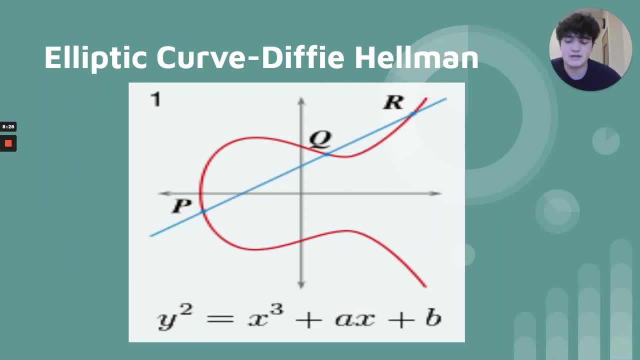 Alice and Bob would, with an elliptic curve, instead of raising the generator to their private key, that is, g to the power of a or g to the power of b, and sending each other those values as public components of the symmetric key, they now multiply the generator by their 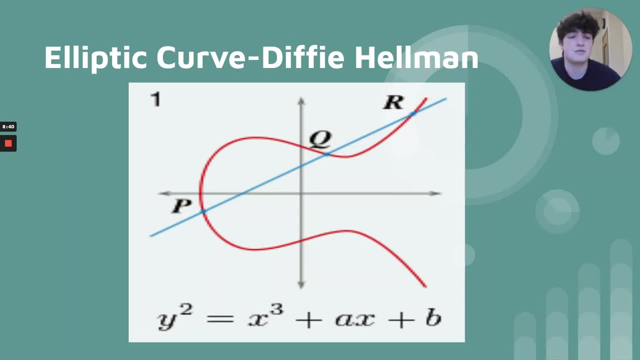 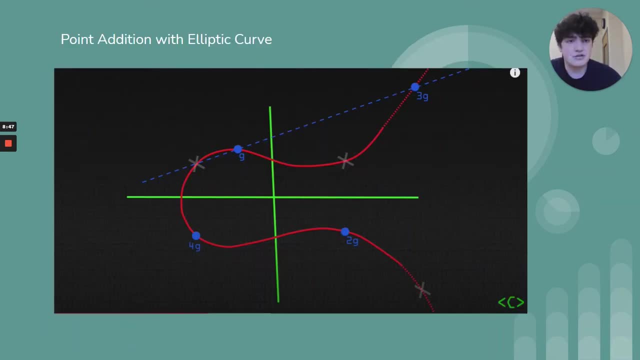 private keys a and b respectively in a process known as Poisson-Hellman. So how does point addition work with an elliptic curve? When we add a point g to itself, in other words g plus g, we simply take the tangent line at g. 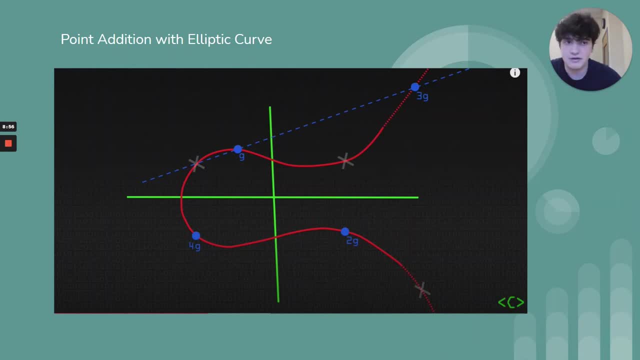 along the curve and find the other coordinate at which it intersects the curve, then find the reflection over the x-axis and that becomes 2g. If we wanted to find 3g, in other words g plus 2g, we'd take the tangent line between 2g and g, find where else it intersects the curve. 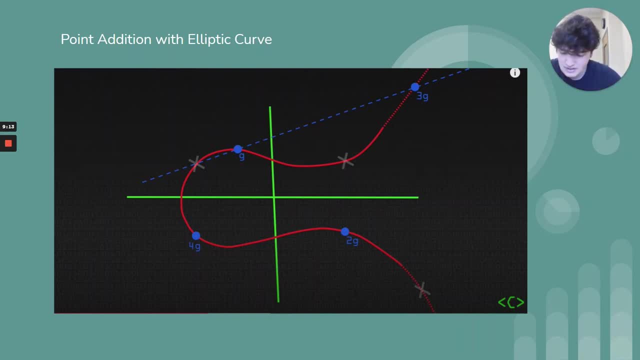 and then reflect it over the x-axis. In this way, instead of randomly jumping around the clock face as we did in Diffie-Hellman, we are moving around the elliptic curve seemingly at random. In Diffie-Hellman, the trapdoor function meant that an adversary could get hold of the public. 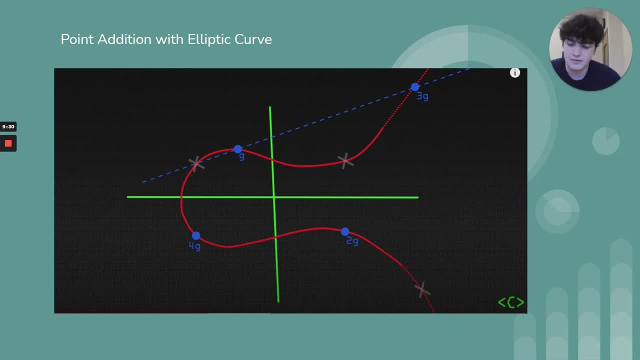 components of the symmetric key g to the power, a or g to the power of b, which Alice and Bob sent one another over public networks. but they couldn't use that product in order to extract the private keys a or b Within elliptic curve. the trapdoor function means that an adversary can get hold of the public. 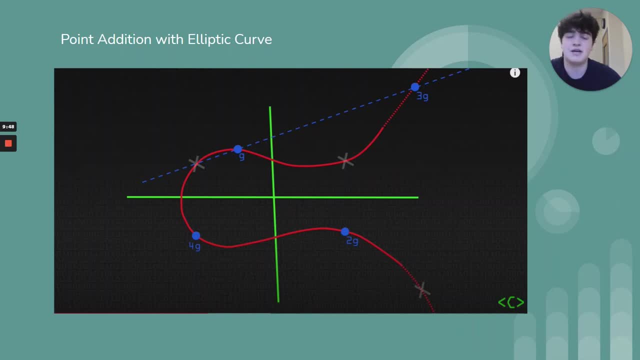 components that Alice and Bob sent to each other, namely g times a or g times b, which are coordinates along the curve, but cannot determine or cannot extract a and b from this, In other words, because we move seemingly at random along the curve when doing point addition. 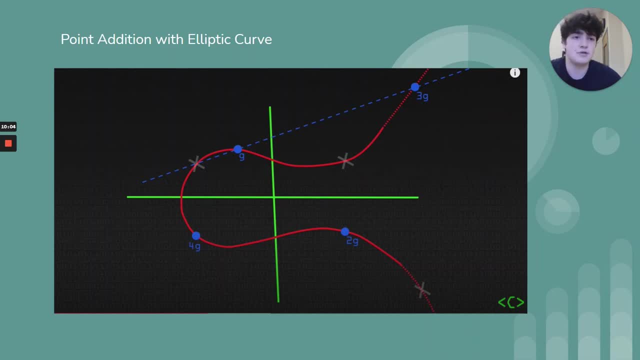 we cannot look at a point and determine how many additions or steps we took in order to get there. Once Alice and Bob receive the public components that they have sent to one another, they multiply these components. they multiply the components of the symmetric key that they have sent to one another. they multiply these components by their 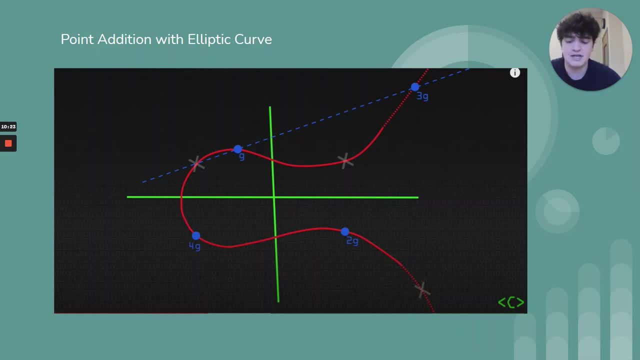 private keys and both end up with the same symmetric key, namely g times a times b, which is another coordinate along the curve. Once again, Alice and Bob have essentially created a symmetric key together by sending each other public components of this key from which the private keys could not be extracted. 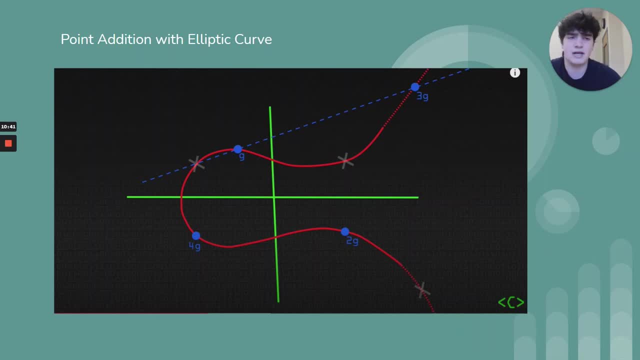 So you might ask, why add this unnecessary complication to Diffie-Hellman? Well, as it turns out, elliptic curves are much more efficient than the Diffie-Hellman key exchange, because we can get away with much shorter key sizes using this method. On the flip side, however, some mathematicians are skeptical of 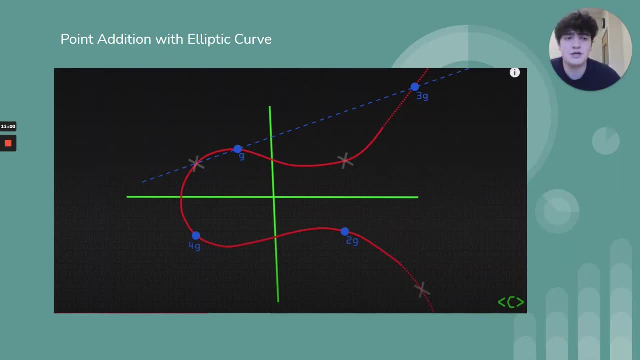 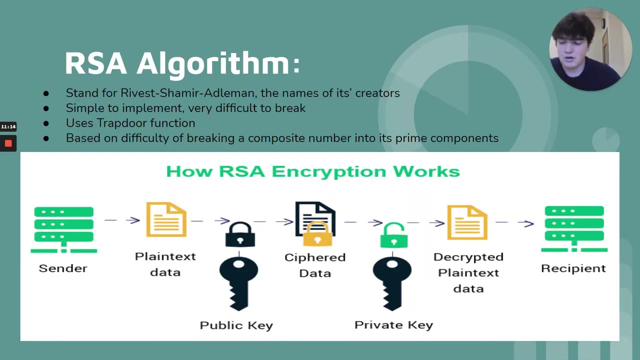 elliptic curve cryptography because in the past, backdoor approaches to break the system have been found. For this reason, we now turn our attention to an extremely successful crypto system which has been proven to be unbreakable over the past decades, known as RSA. RSA stands for Revest. 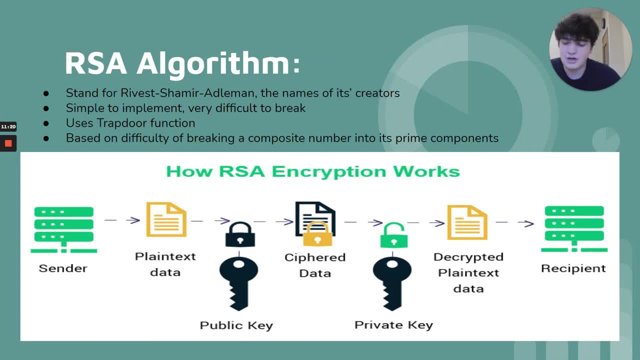 Shamir and Adelman, who are the creators of this crypto system. What makes RSA so special is that it is simple conceptually and simple to implement, while nearly impossible to break. What do I mean by this? RSA is based on a simple idea in number theory. the difficulty in breaking a composite. 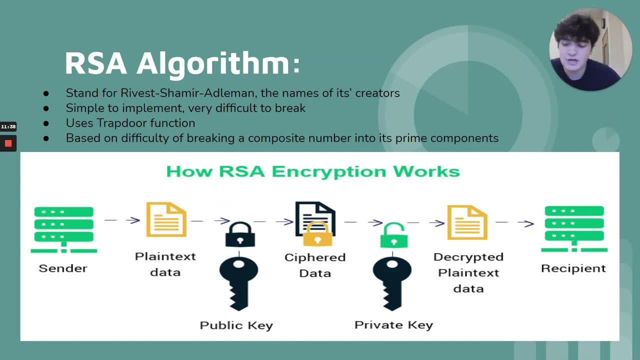 number into its prime components, Without knowledge of these components beforehand, of course. Additionally, being a public key crypto system, RSA is very nice for a situation where there is only one primary recipient, For example in a PayPal transaction where we are sending money to one of our friends. So how does RSA work? 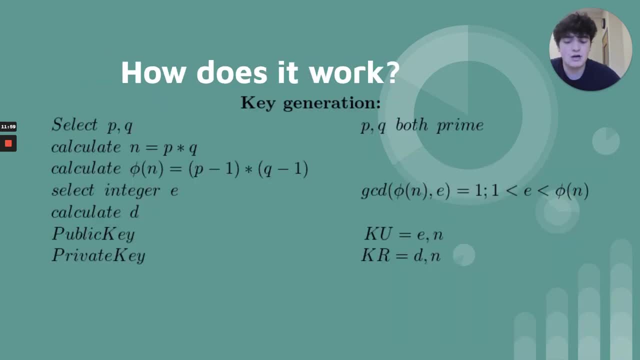 Each user of the system first chooses two extremely large prime numbers over hundreds of digits long. Let's call these values P and Q. Then P and Q are the primary recipients of the product N. Then they use a special function known as the phi function in order to work out how many. 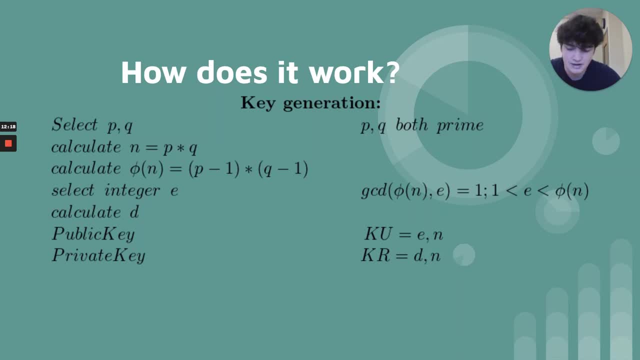 natural numbers less than N are relatively prime to N, Which just means that they share the greatest common divisor of 1 with N. This is given by the simple formula: phi of N equals P minus 1 multiplied by Q minus 1, which we can see on the screen. Next, the user chooses an encryption key. 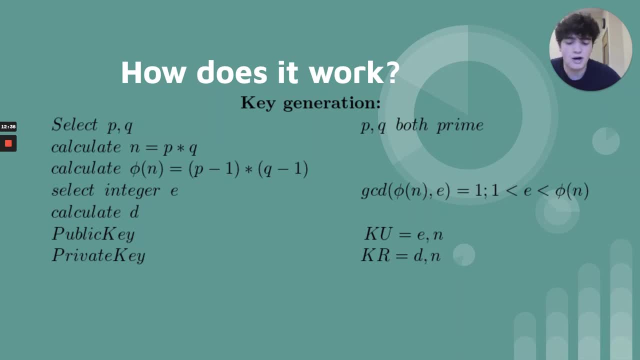 which we will call E. that represents some number between 1 and phi of N. This is a very simple function that is relatively prime to phi of N. This being relatively prime to phi of N, it means that the multiplicative inverse of E exists. So, in other words, if we have E, we can get the decryption. 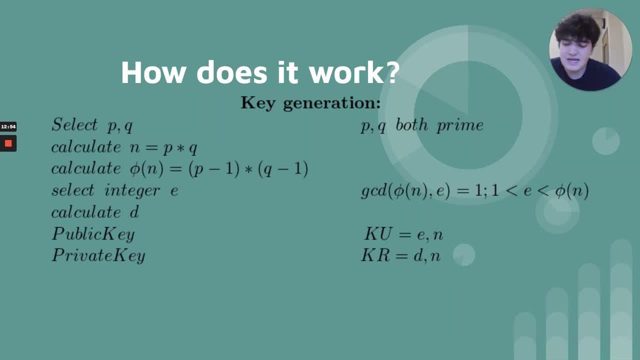 key as well. This means that E multiplied by D is congruent to 1 modulo phi of N, which will be important for later. Note that each of these values- P and Q and E- are randomly chosen via a random number generator that uses a random number generator, So this is a very simple. 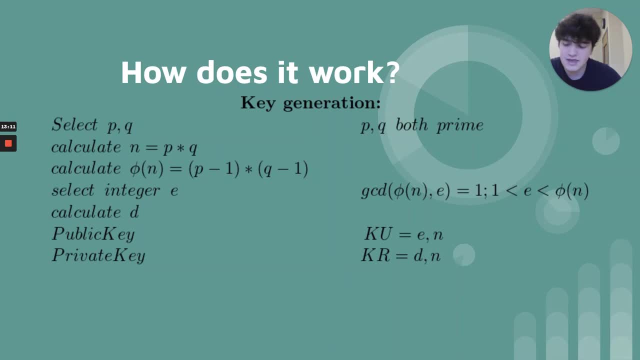 function that uses statistical properties of a truly random sequence. Then the encryption key becomes N, comma, E, So just N and E, Which is released to the public and can be accessed by anyone. The decryption key D, on the other hand, must be kept private by the user, as obviously it. 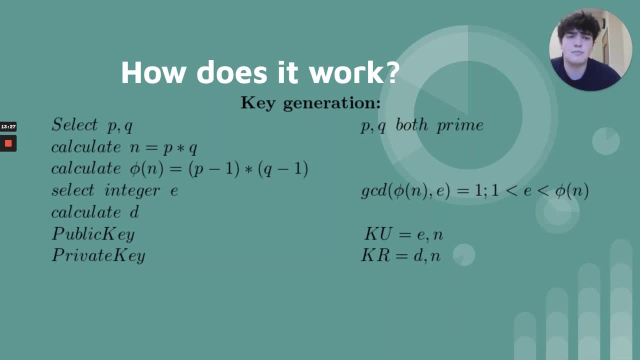 is the key to unlock the encrypted message. So now let's explore what makes this algorithm so special. Suppose that we have a message which has a numeric value P. If Alice wants to send this message to Bob, she raises her message to Bob and says that the decryption key D is the key to unlock the.